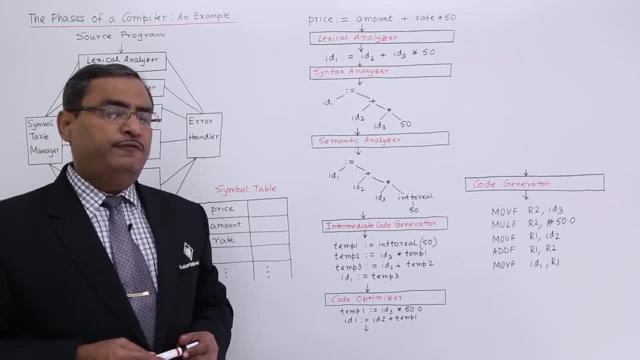 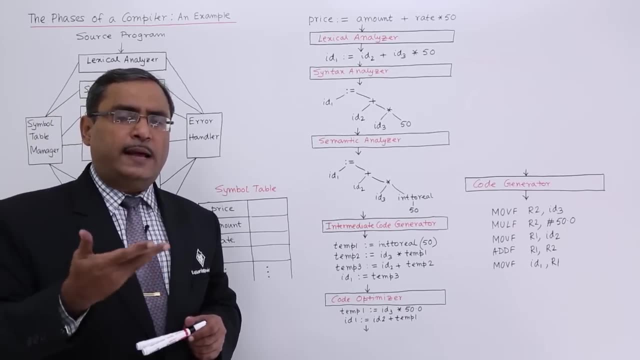 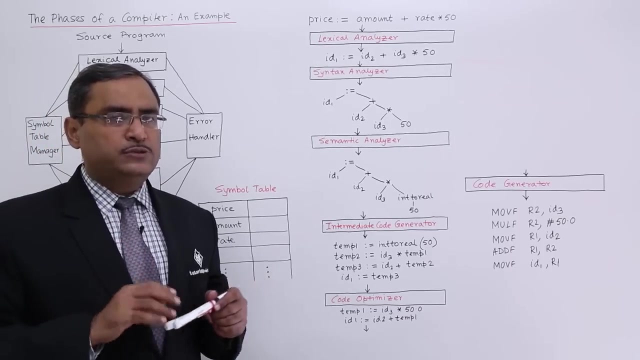 colon equal to Amount plus rate into 50.. Let us suppose this price, amount and rate are of the type real. that means they can have some fraction part And this 50 is purely in integer. ok, So just keep this one in mind. we will be taking care of that issue. So lexical analyzer will take this. 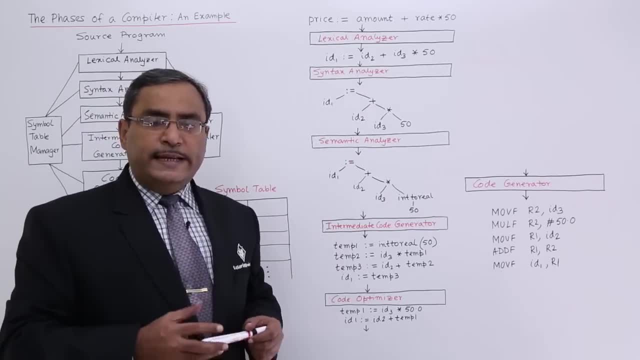 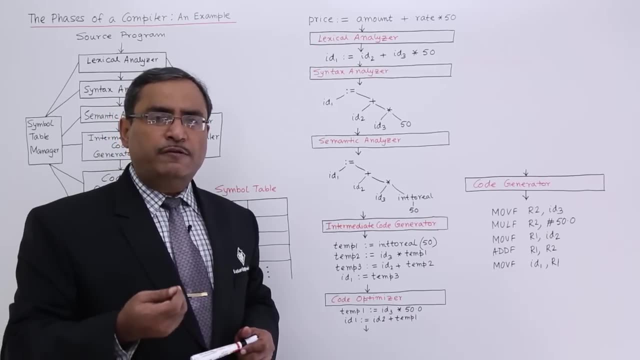 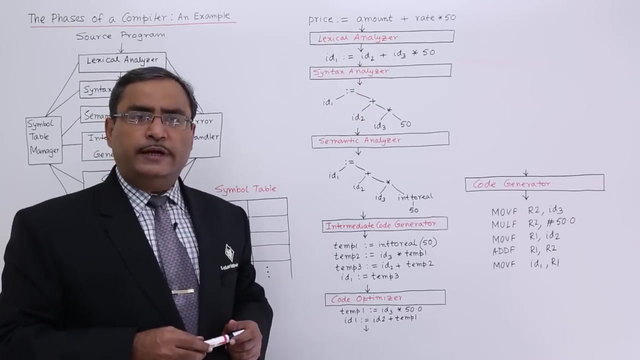 particular statement as input and it will produce the series of tokens as output. So it is producing. this price will be detected as identifier 1, identifier means variable, So identifier 1 and this colon equal to. is this one, Then amount has been detected as your say. 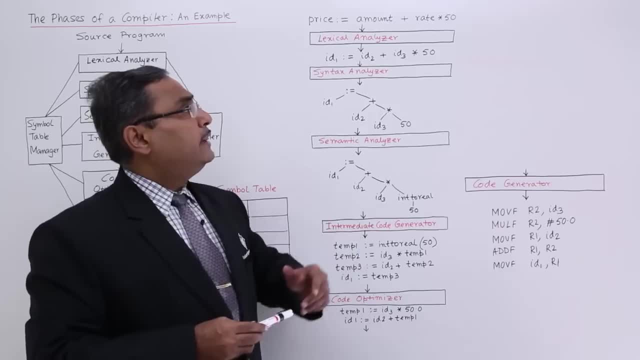 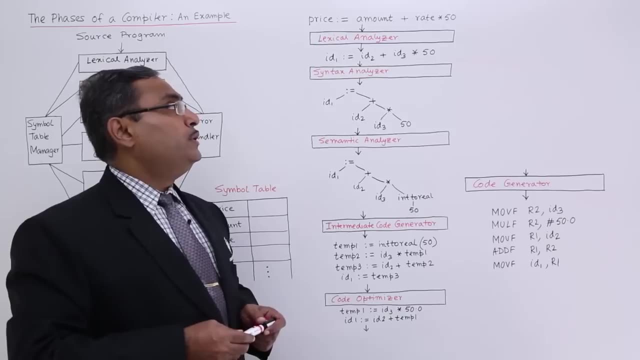 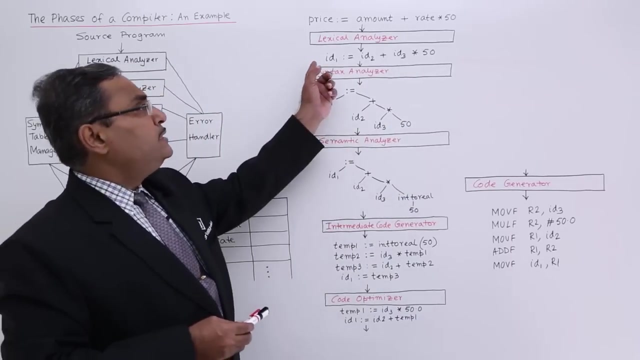 identifier 2 plus has been kept as it is And then rate has been detected is another variable, So it has been detected as identifier number 3, into is there and there is another integer data, 50. So it is taking 50 as a constant. So this is the output of the lexical. 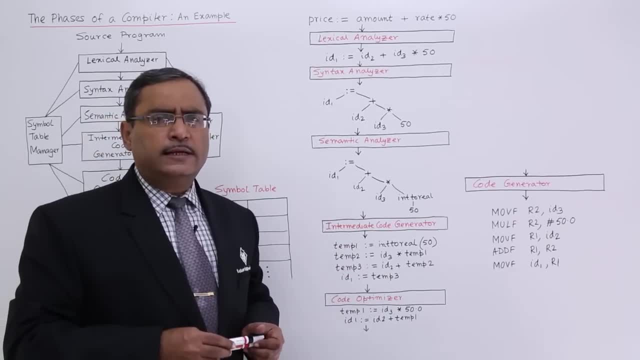 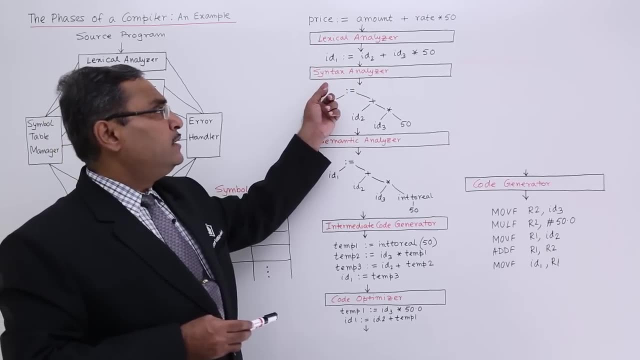 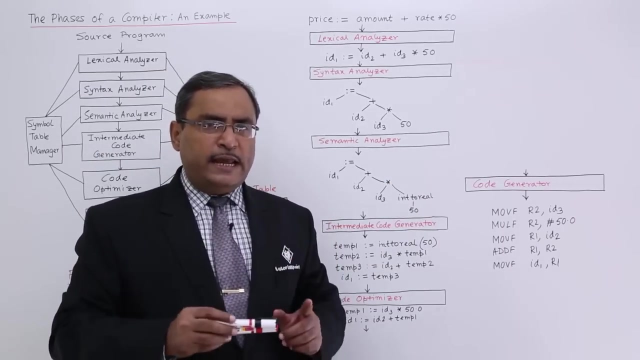 analyzer. ok, different lexical analyzer can interpret this line in different way. ok, now it has come to the syntax analyzer. syntax analyzer will check whether this tokens are in the proper order or not according to the grammar. so each and every language- programming language, high level language- should have some dedicated grammar, and the grammar will be: 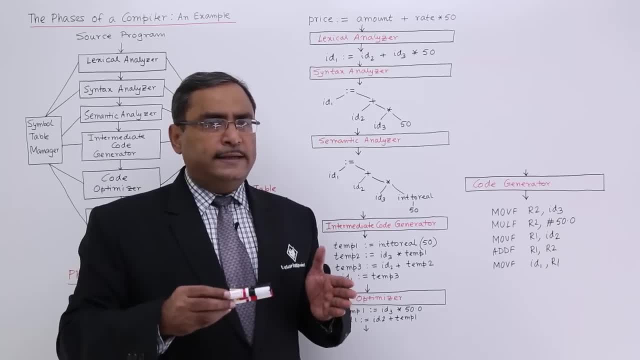 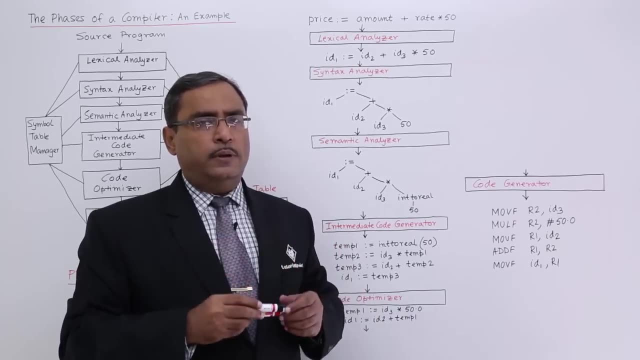 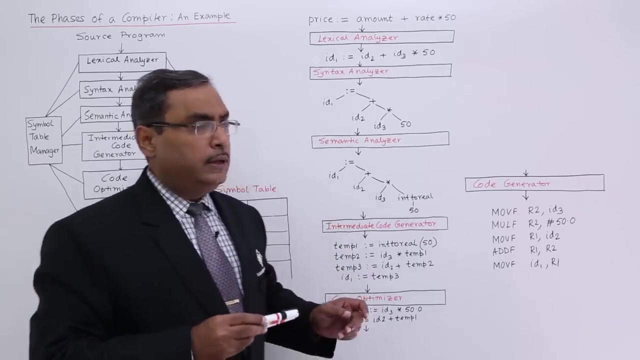 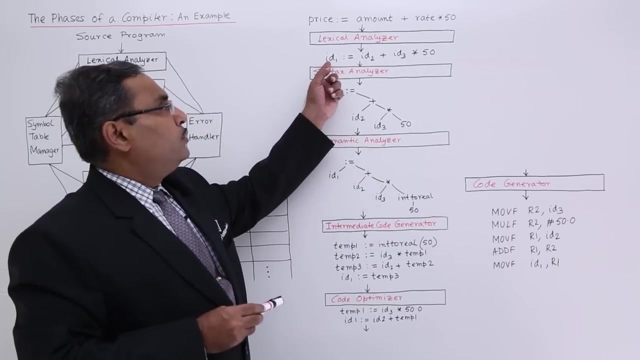 having set of production rules. so as a result of that, it will check whether all this tokens are in the proper grammatical, according to the grammar maintained by the language, if the sequence according to the grammar or not. so to check that one, it will construct one parse tree, so this is known as the parse tree. so now it is doing in this way, so it is my. 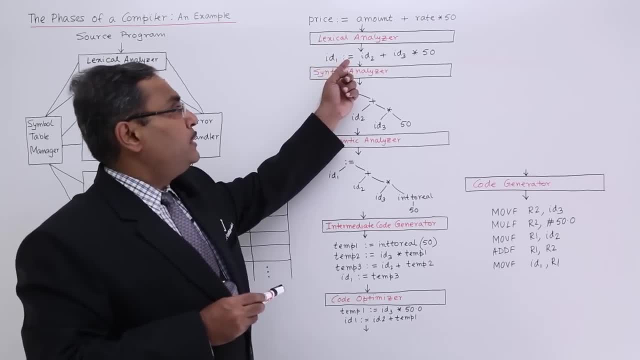 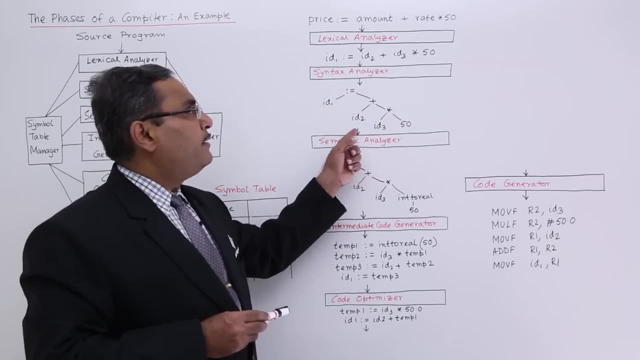 left hand side. this is my colon. equal to that is the assignment operator and this is my right hand side, so it will doing this way. so this is assignment operator. left hand side is id1 and this is my right hand side. right hand side is a variable. right hand side is: 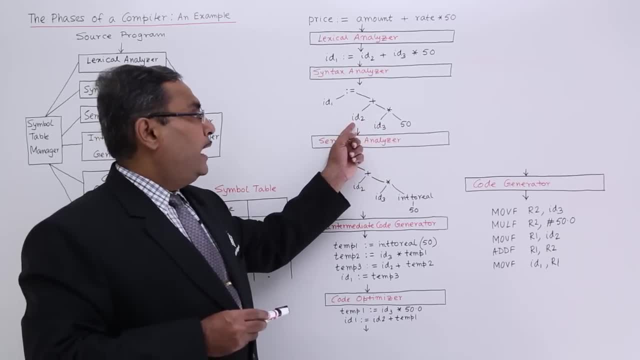 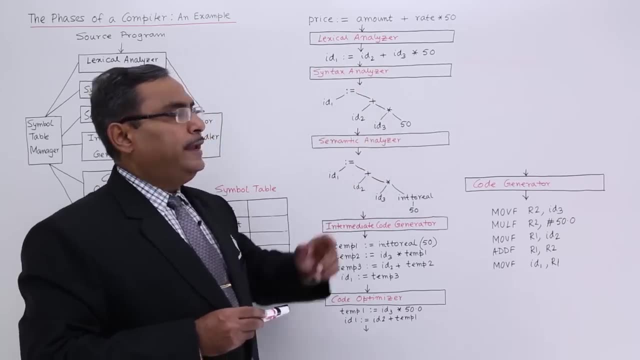 having id 3 into 50, id 2 plus. So now it will be done in this way. So id 2 plus id 3 into 50. So now it has been done in this way, It will be done by the lexical analyzer. 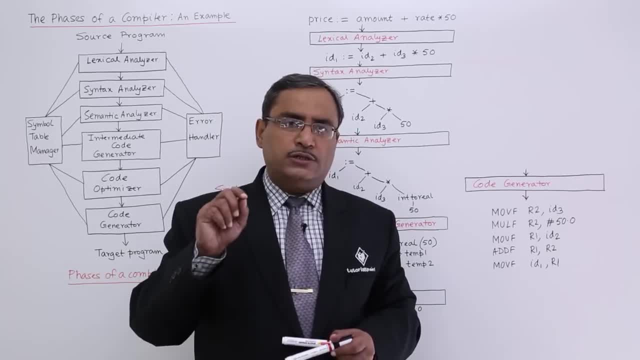 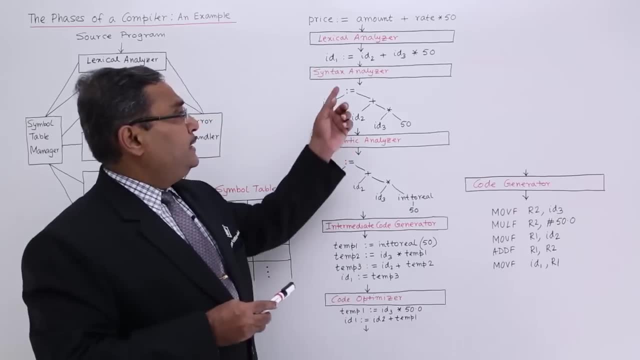 If lexical analyzer finds that tokens are in accordance to the grammar of the language, then it will parse it. Otherwise it will produce the syntax error. ok, So syntax analyzer will form this parse tree. So parse tree can be constructed from the top down approach. 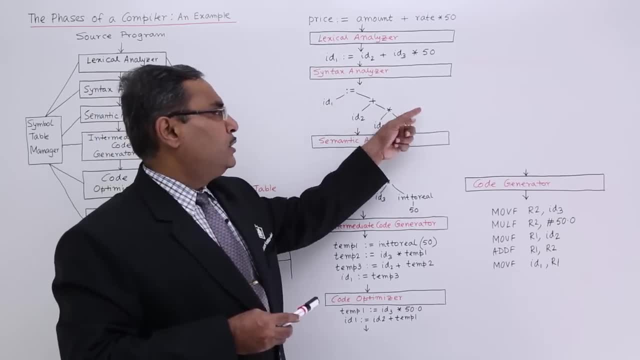 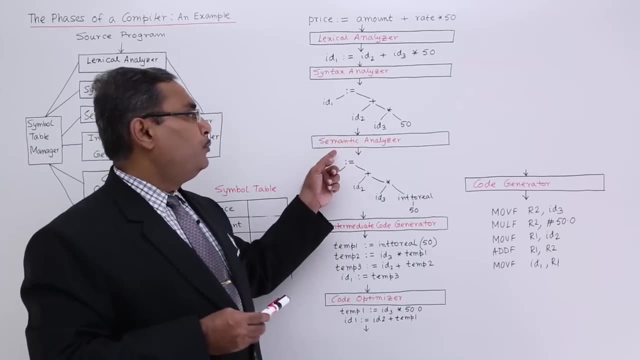 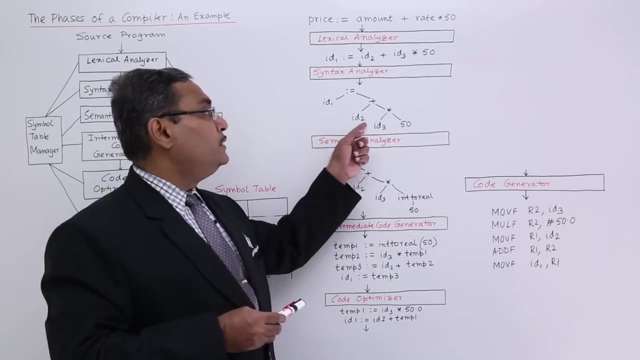 or in the bottom approach. whatever it is, If the parse tree construction has been completed successfully, that means this particular statement is syntax error free. So now it will come to the semantic analyzer. So 50 was in integer, but this variables. 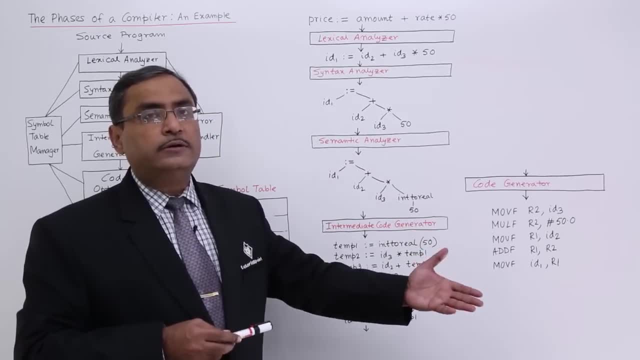 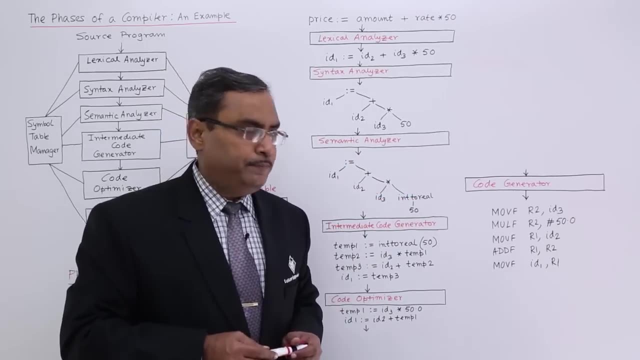 identified were where of the type real data type. So that is why integer to real conversion will be done by the semantic analyzer. So it will change the meaning of this 50. So auto type type upgrade will take place. So now intermediate code generator will take this one as input. 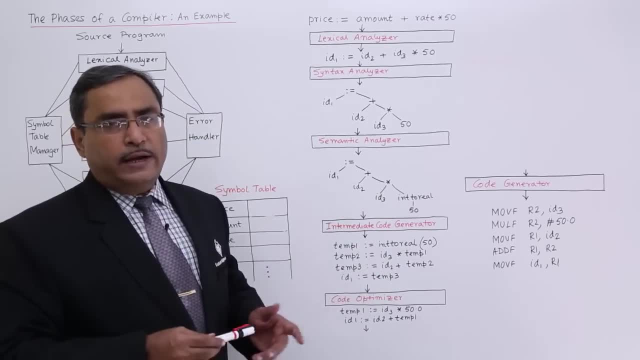 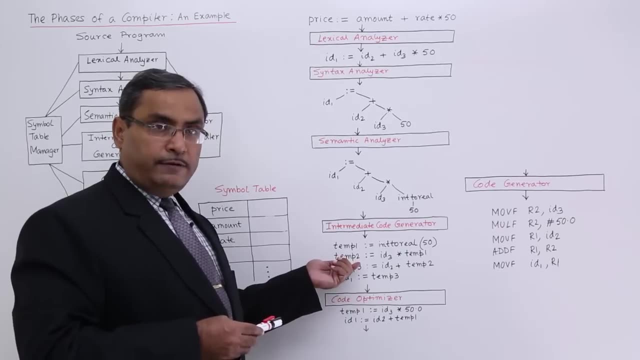 and it will produce the statement in some different format. here they have used the three address statement, So we are having three addresses maximum. So this is the target address for the target. this is the addresses for the source, So it has been mentioned. 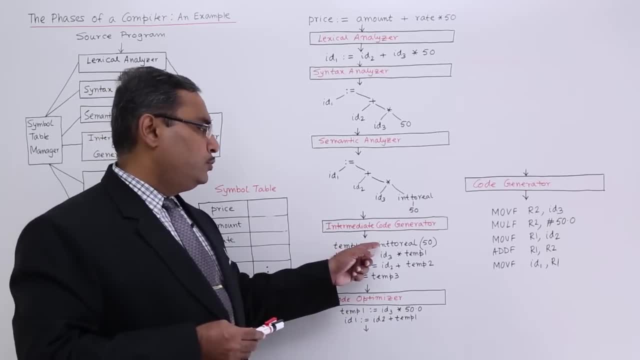 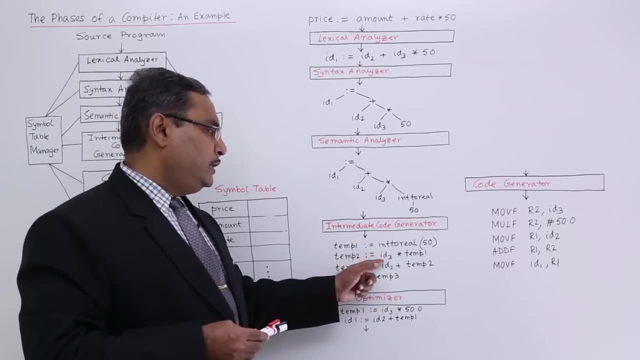 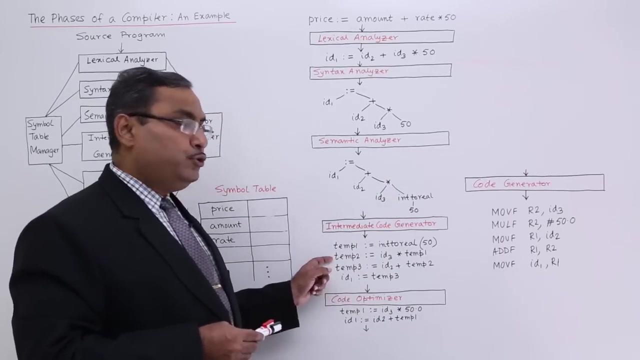 this one in this way. So temp is equal to colon, equal to integer, to real 50. So it will be. the code will be written in this way internally: So ID3 start temp 1.. So temp 1 means 50 actually. So ID3 start temp 1 will be assigned to temp 2 and this temp 2. 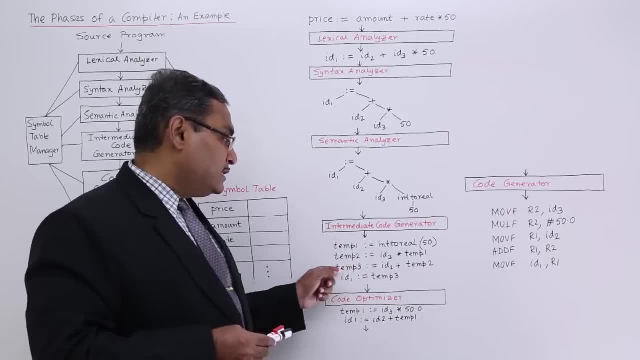 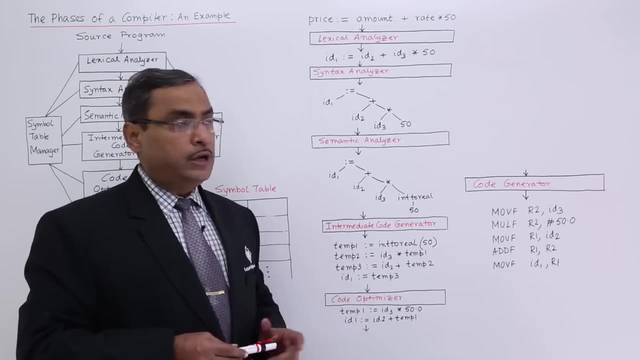 will be added with ID2, and that has been kept in temp 3, but it will be assigned on to the ID1.. So ID1 Assignment Operator, temp 3.. So this is my intermediate code generator, So it will be taken as input. 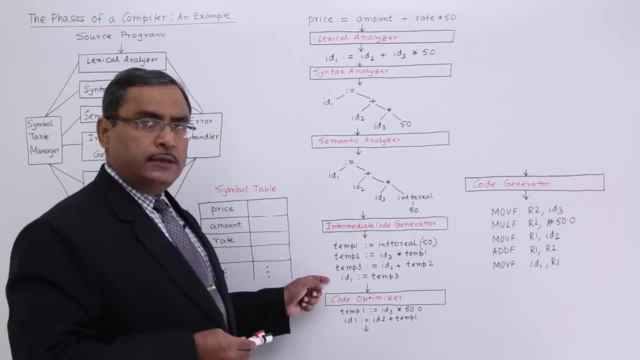 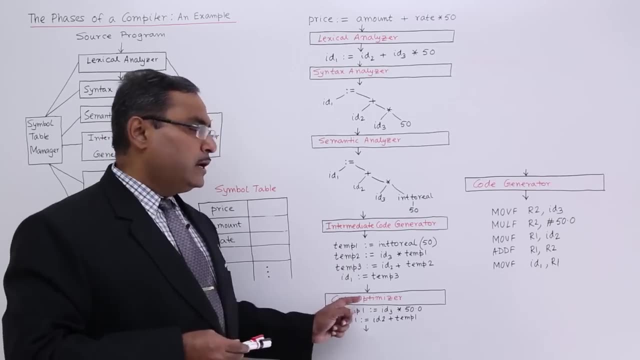 by the code optimizer. So there are some redundancies here. So 1,, 2,, 3,, 4- this 4 statements can also be expressed in the form of this 2 statements and that will be done by the code optimizer. So it will bring some optimization of the code. 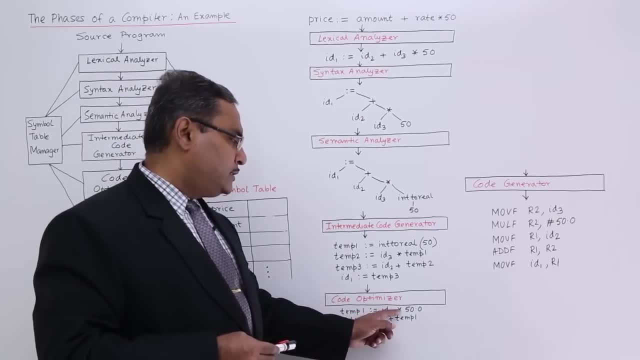 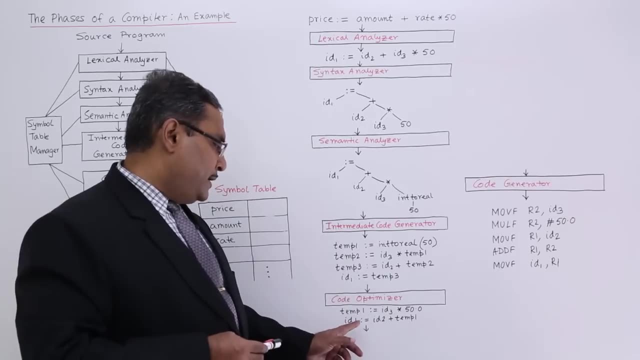 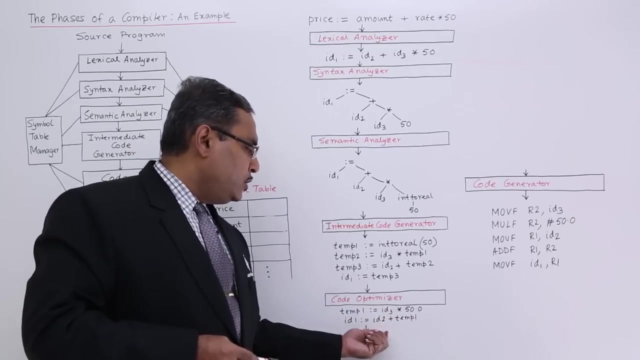 So temp 1 SME operator. ID 3, star 50.0.. So it has been converted to real. that means it is. it can have the fractional part and this temp 1 is containing this part, this part. So as a result of that, you can go for this addition. So ID 2 plus temp 1 will be assigned. 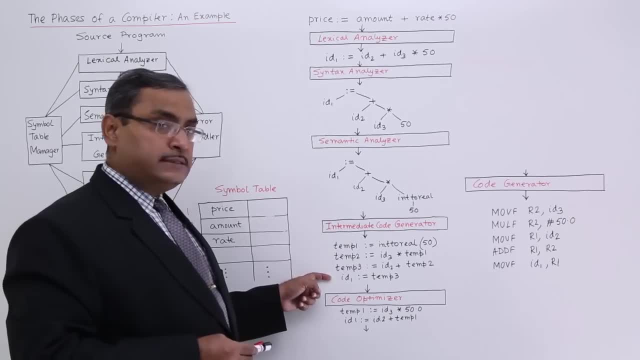 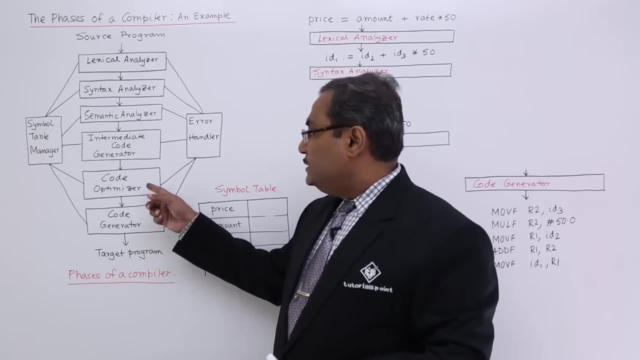 to ID 1.. So you see this: 4 statements have got reduced to 2 statements, and that has been done by the code optimizer. So after code optimization we are having the last phase remaining, that is, the code generation. So this particular thing will be taken as input. 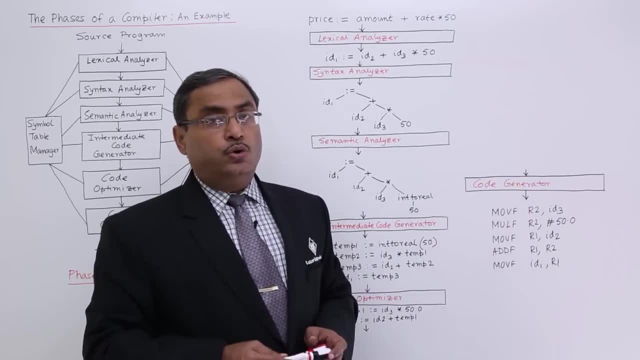 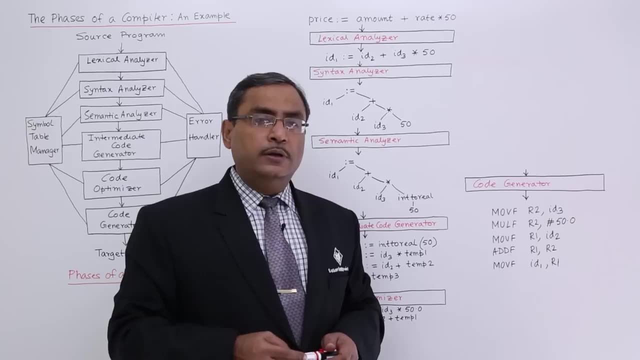 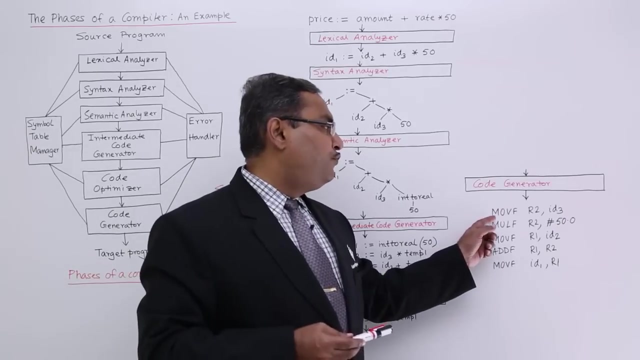 by the code generation. So code generator. So code generator will convert it to the respective registers number, Number or registers name which is available in that particular architecture, depending upon the target machine of the target program. So it is going for move f, that is float. 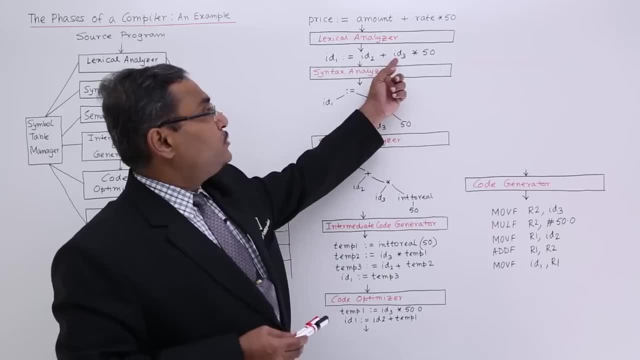 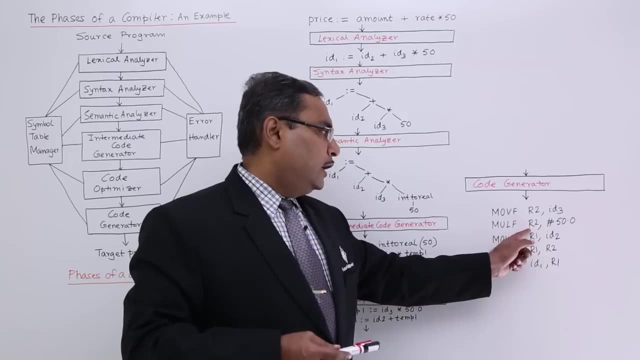 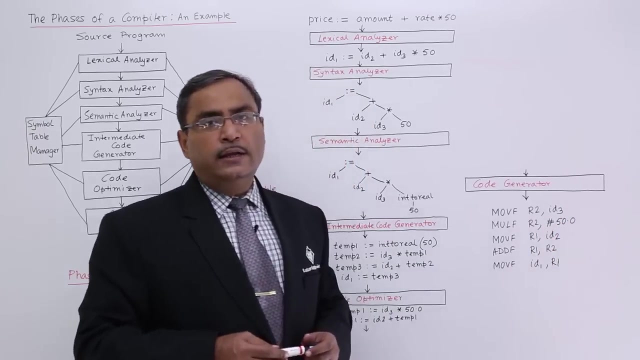 Move float R 2, ID 3.. So ID 3 means this one. So this one is getting moved to R 2.. Multiplication float mal f R 2 star hash 5.0 for 50.0.. So that means this hash is indicating that. 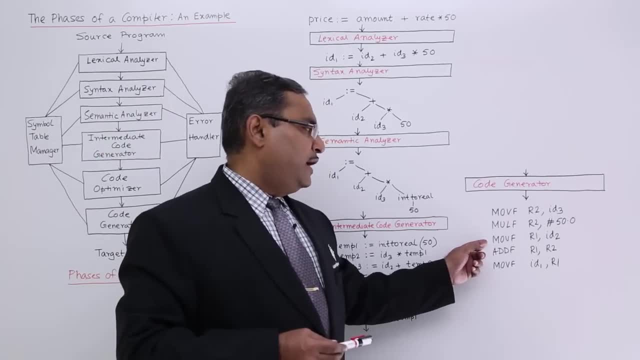 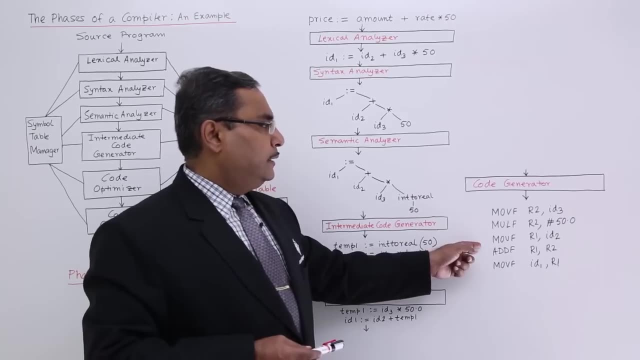 it is the real type of data. So now move f. So move float R 1, ID 2.. So now ID 2 has got moved to R 1 and the multiplication is: result is now still remaining in R 2. So 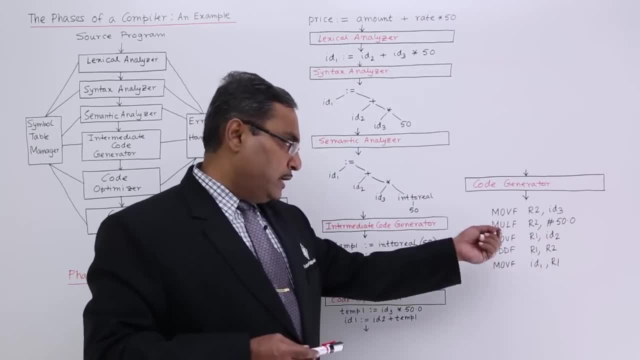 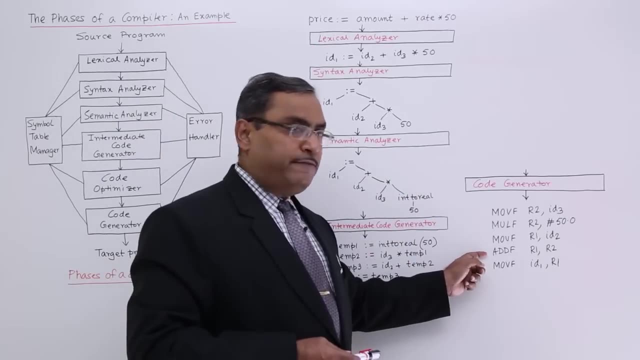 move f R 1, ID 2.. So ID 2 has come to R 1, R 1 is containing ID 2, R 2 is containing ID 3 into 50. So add float R 1, R 2.. 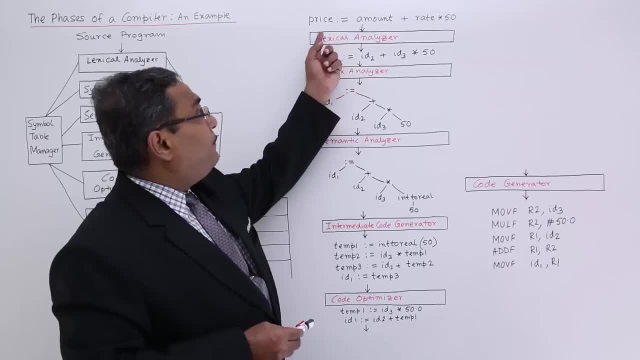 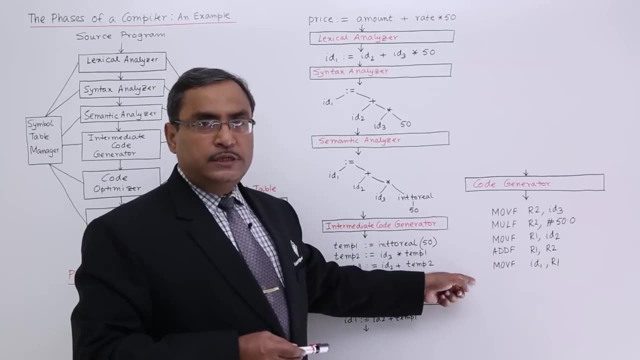 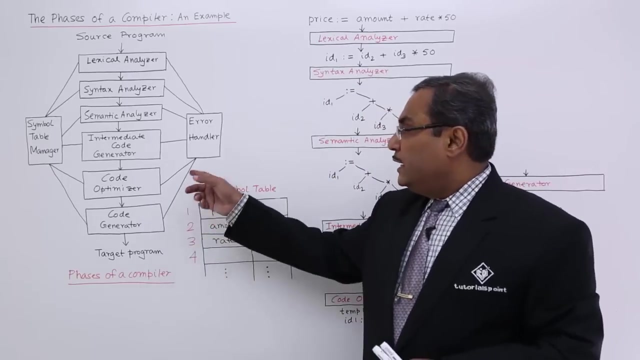 in r1, but the sum should be kept in id1.. So move float id1- r1.. So this is the code generated. This is the generated code for the target machine, depending upon the architecture of the target machine. So here, in this particular process, this particular 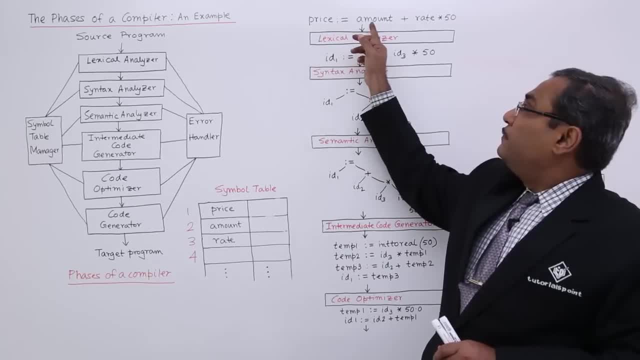 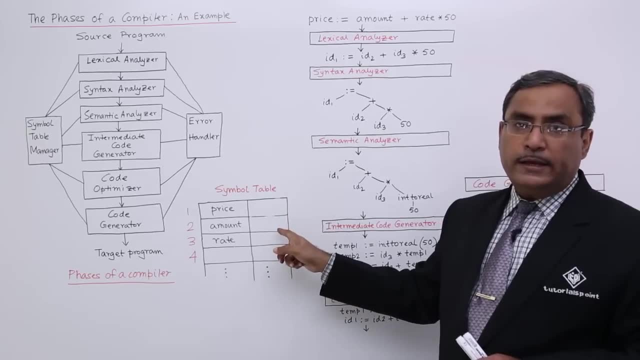 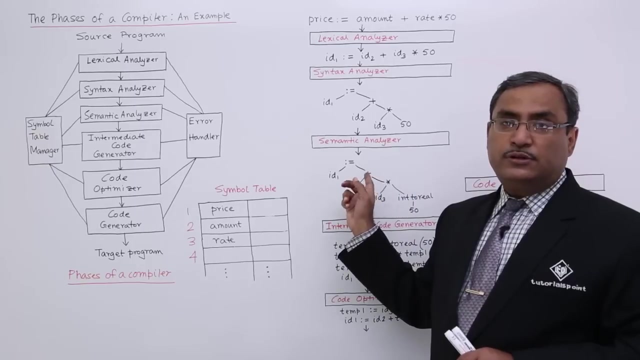 symbol table will get generated. So here we are having three variables, So the respective symbol table will be marking them. So it will be doing the book keeping here. So price, amount and rate, So there is a symbol table. So if the program during execution finds 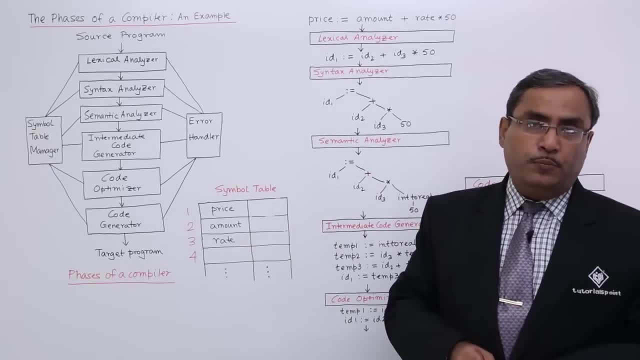 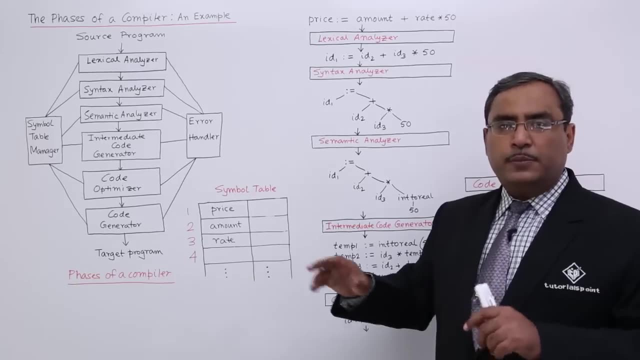 that these variables are not defined, then obviously it will produce a error message. So this is the symbol table which will be doing the book keeping. So there is a data structure. we will be having a separate video on the symbol table later on. So price amount.